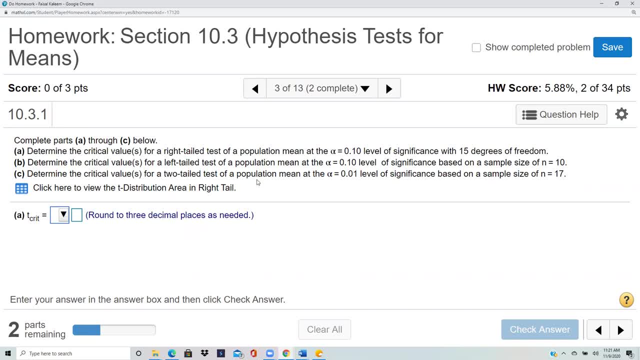 we are not now dealing with hypothesis testing for means. So in the previous section we were dealing with hypothesis tested tests for proportions And so in that case for critical value we were using a normal calculator. When you are dealing hypothesis test for mean, you do t calculator for the critical values. 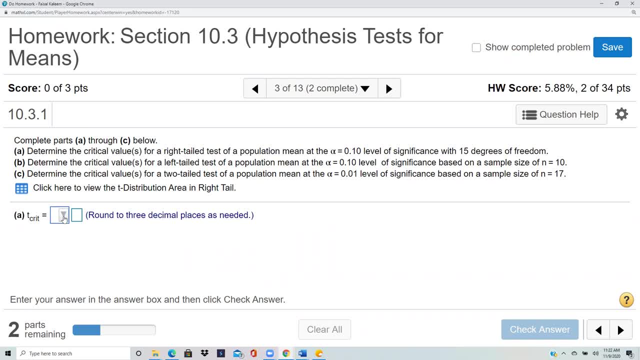 So remember critical values. one of the three calculators has to be used. For proportion stats, we use normal calculator. For I mean for proportion hypothesis or percentage hypothesis, we use normal calculator, And if the hypothesis test is testing means, we use t calculator. In this particular, 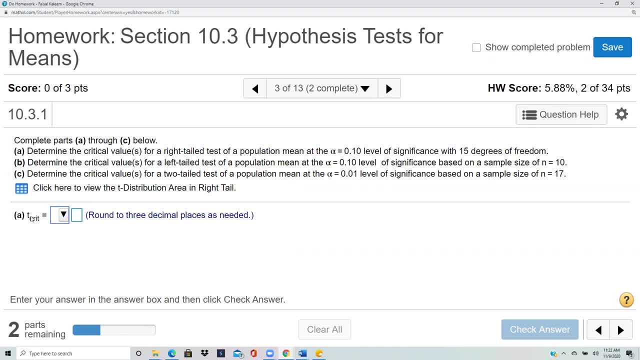 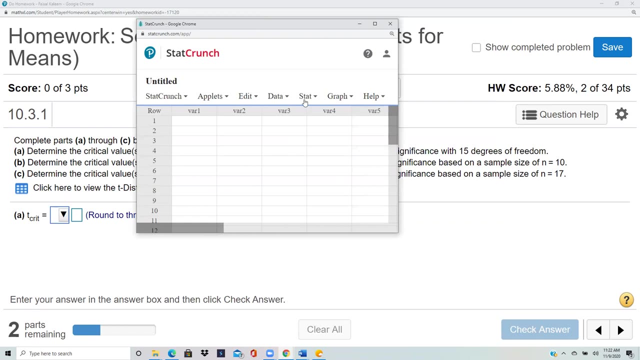 problem. they don't mention any hypothesis but they are just saying to find the t critical value, So that's obvious that you have to use t calculator. So stat crunch, Stats calculator, t, So degrees of freedom, is needed. That's 15 for part a And if it's a right tail test. 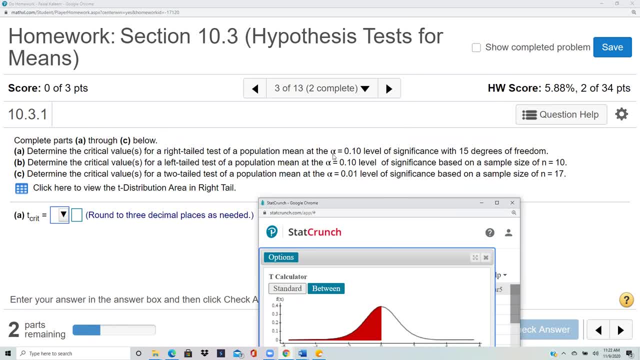 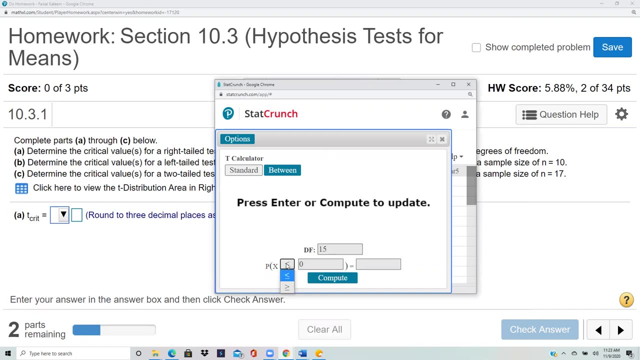 you put alpha In the right tail. alpha is the area, Tail area. So you put the tail area of 0.10.. Decrease of freedom is 15. And make it right tail So greater than And the area was 0.1.. 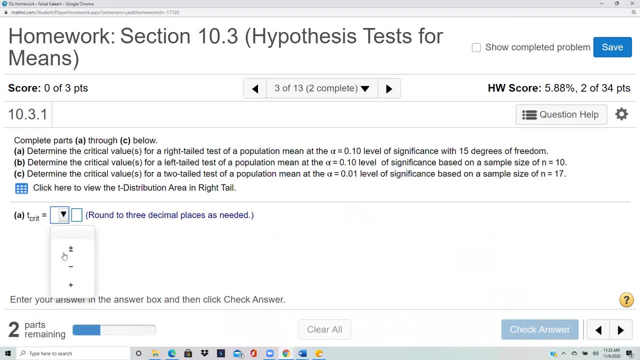 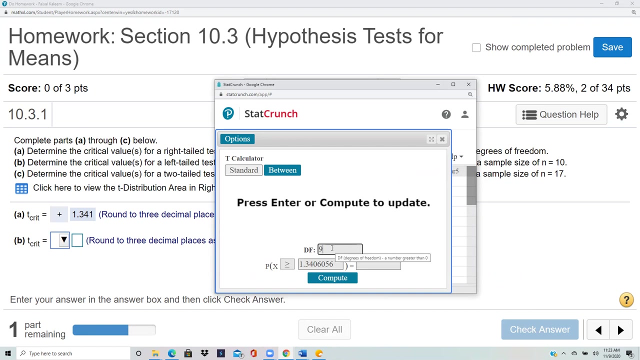 So 1.341 positive. And then You have a left tail. alpha is again 0.1.. And this time sample size is 10.. So degrees of freedom will be 9.. 1 less than the sample size. In the previous problem they gave degrees of freedom, so you just put them as such.